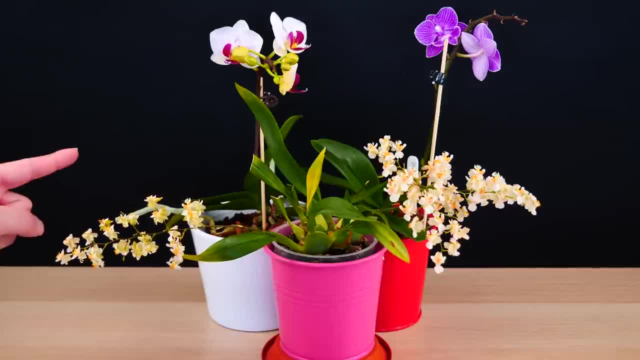 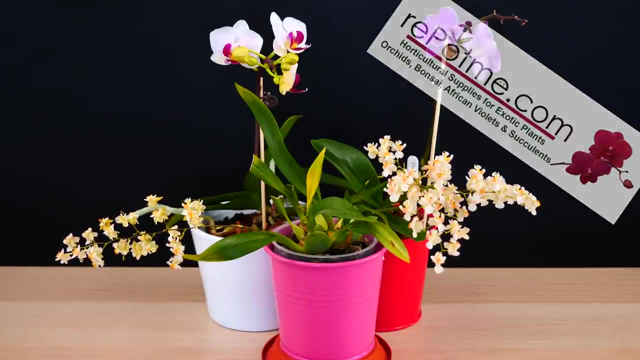 a lot of useful information planned for you guys, so stay tuned for that. And before we start, let me thank repotmecom for sponsoring this episode and this entire series as well. Repotme offers you everything you could need to properly take care of your orchid, from potting medium to. 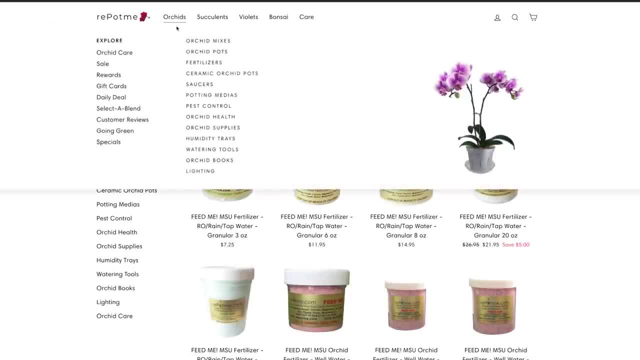 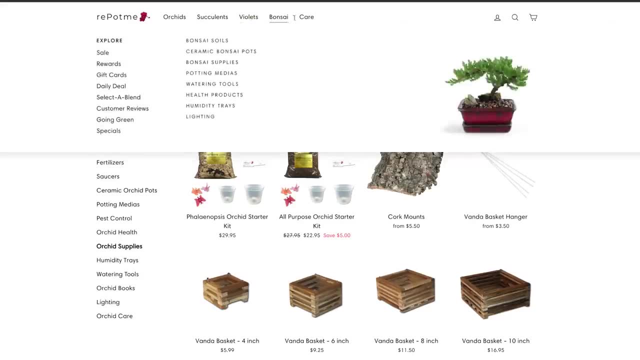 pots, fertilizers and all sorts of accessories, And many of the accessories you'll see me use in this series and in my videos are actually provided by them, So I'll link it down below to their website and to the products that I'm gonna use. Feel free to check them out at any time and with 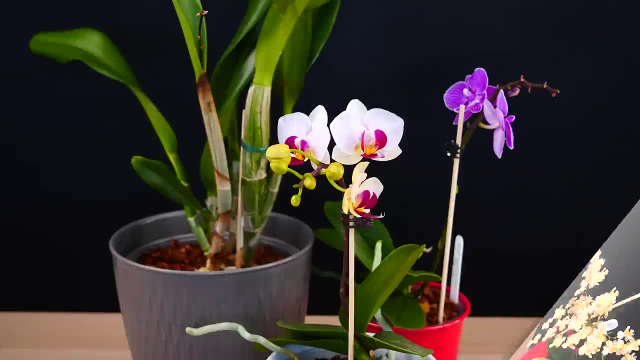 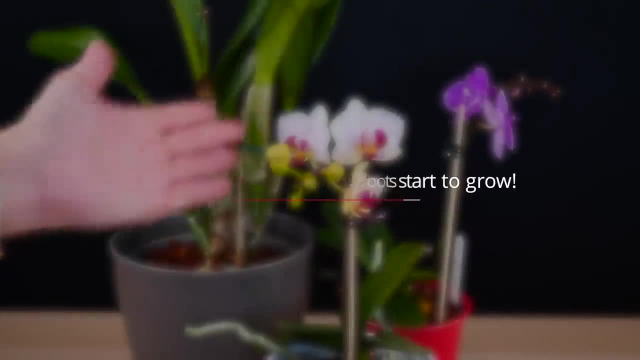 that said, let us get on with the subject. Tip number one: repot your orchids when you see new roots starting to grow. Now, this tip will not necessarily apply to the Phalaenopsis. Last year we talked about how to properly repot Phalaenopsis. 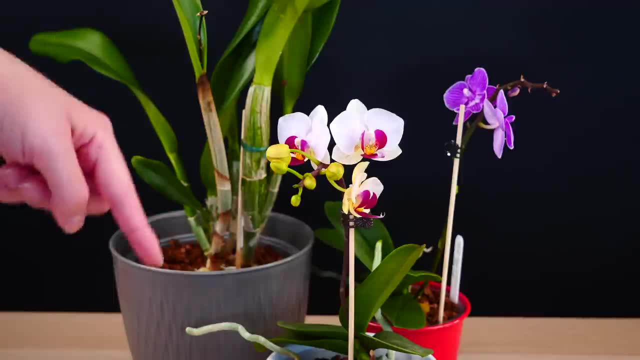 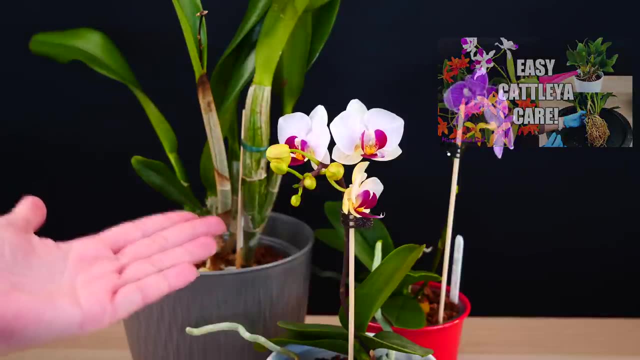 orchids. so if you're interested in this particular orchid, head down to the description or check the info card on the screen to learn more about them. But, as we discovered in our previous care tutorial, on the market we can find many other orchids which we can grow in our homes, such as Catleas. 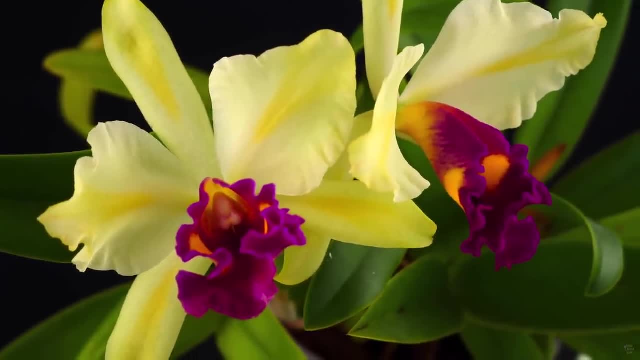 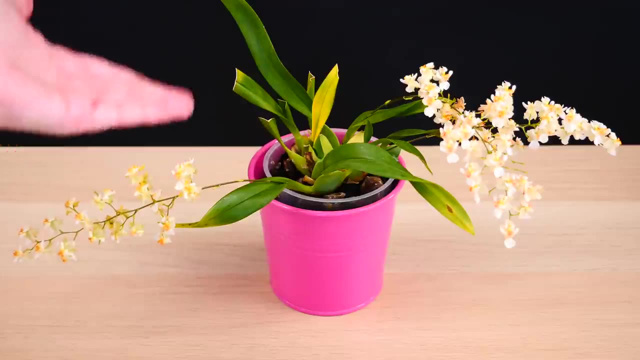 Oncidiums and so on. Those orchids are very different from Phalaenopsis and this tip applies to them in particular. Sympodial orchids such as Catleas and Oncidiums don't have a central stem from which new leaves. 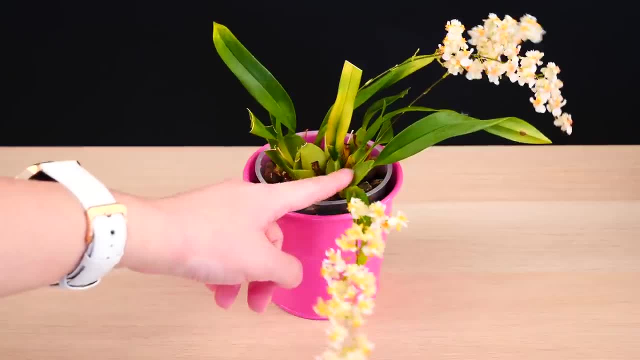 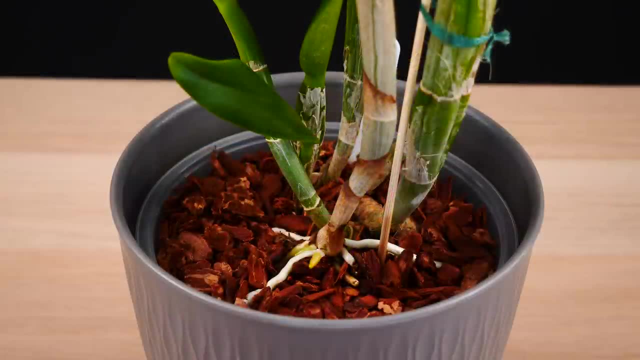 sprout every year. They grow new canes or new pseudobulbs every year And as they grow, these structures will produce a brand new root system. In order to minimize transplant shock, the best time to repot is when you see brand new root tips starting to grow from the base of these. 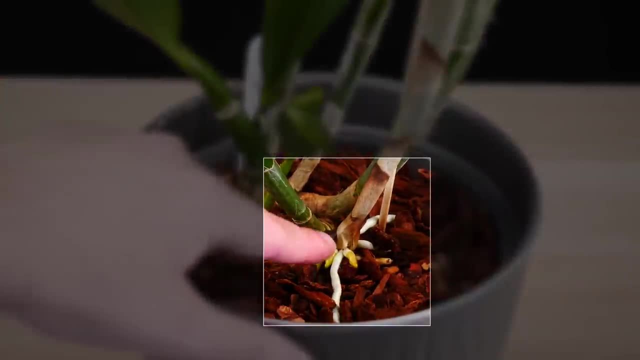 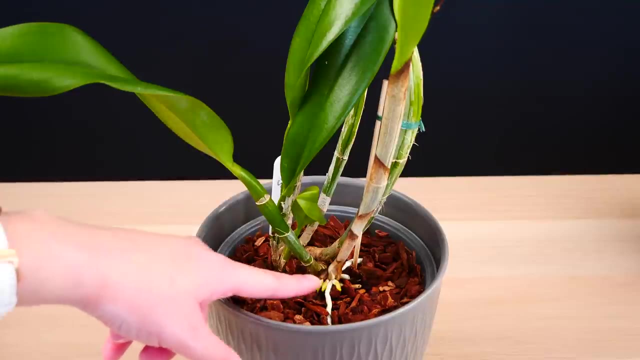 structures. In this example, you can see my Catlea orchid is producing brand new roots from this cane. So if I would want to repot my Catlea orchid, now would be the time, because there is a brand new root system on the way which will make sure that my orchid will stay hydrated and fed. 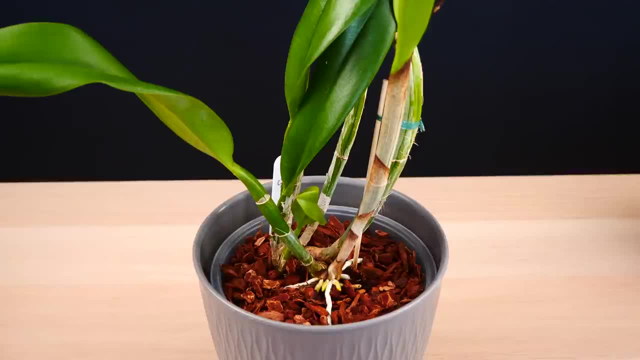 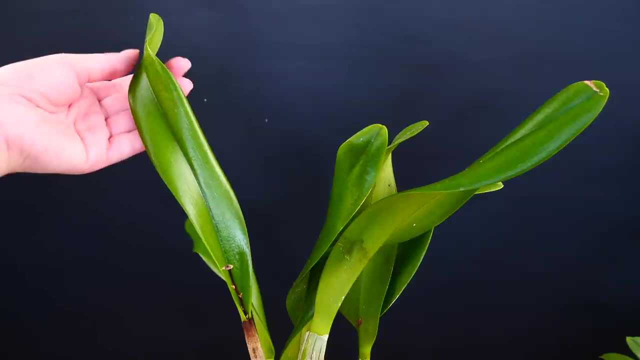 even if the older root system gets damaged during repotting. A little side note: you can skip this rule if your orchid is in serious need of repotting. Maybe the medium is very broken down and it's affecting the roots. maybe you have a pest in the. 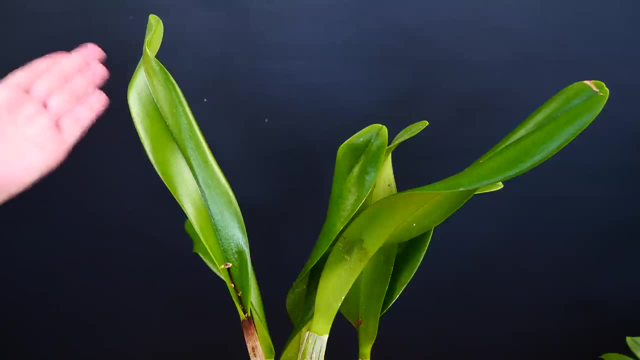 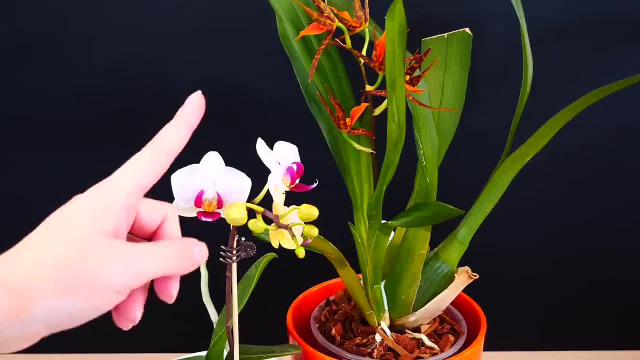 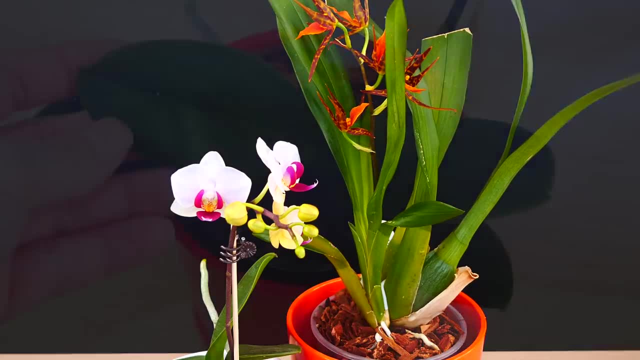 orchid you want to repot. You can repot any orchid you want to repot. You can water whenever you have time in the day. But do make sure that after repotting and watering your orchid, you dry off the leaves, the crowns and the stems, Because water left pooling in these structures. 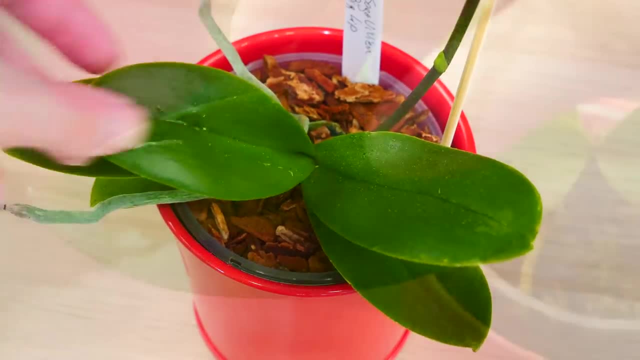 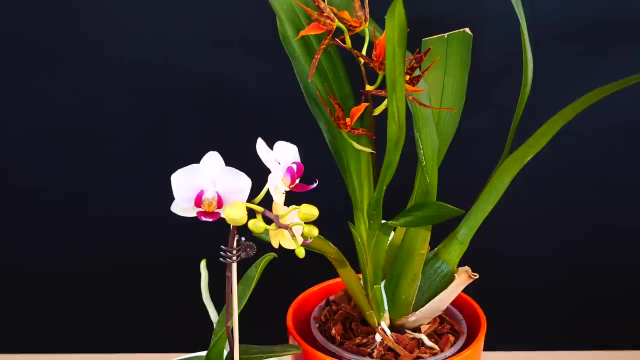 can accumulate pathogens which will damage the tissue and you can end up with parts of your orchid rotting. Our home environments are very, very different than natural habitats. First of all, we don't have wind in our home. Second, we don't have constantly refreshed air. And third, 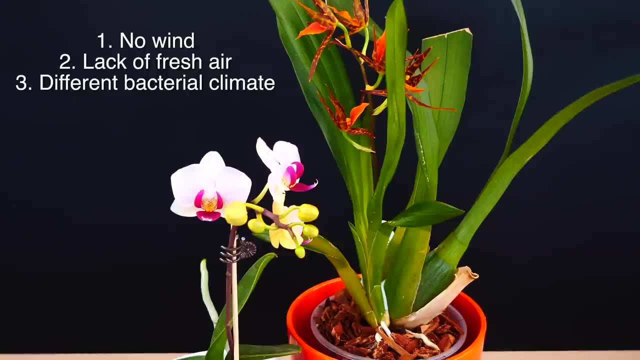 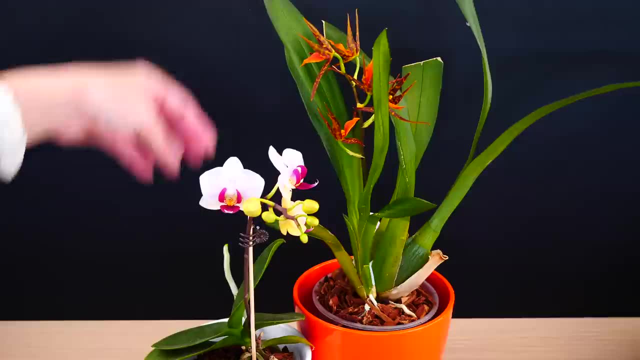 in our part of the world. these orchids might encounter pathogens that they never encountered in nature. It's always better to play it safe and make sure that we don't have any water droplets on the leaves, crowns and stems. If you do get water in the crown of your orchid, get a paper. 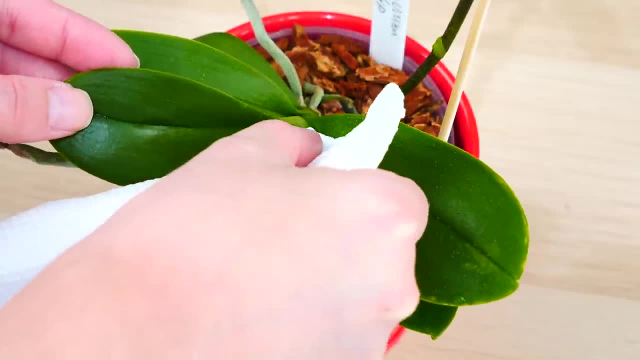 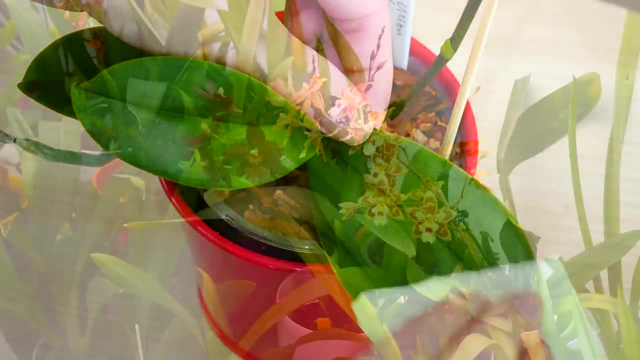 napkin and remove it from the crown As much as possible. try to not keep your orchid in cold temperatures, because they will not favor water evaporation, And if you use a fan in your home, you can actually place the orchid near the fan. 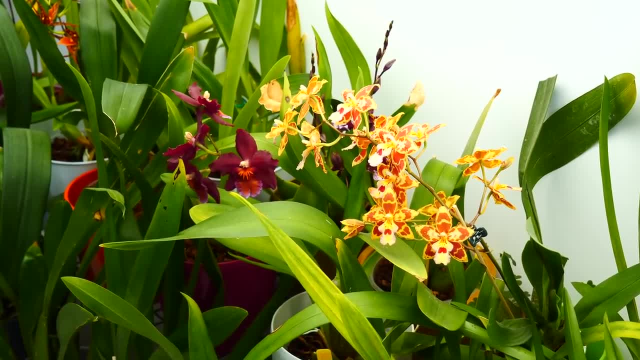 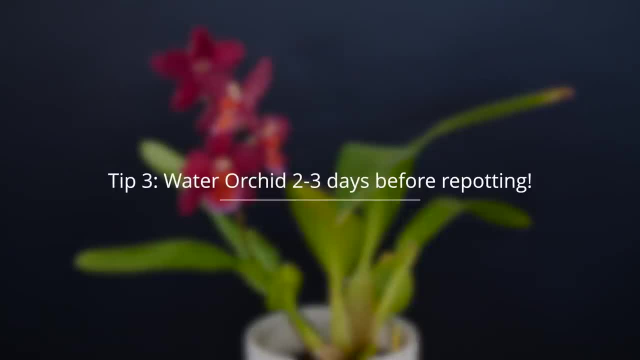 just so it gets a little bit of air movement to help out with water evaporation. Tip number three: Water your orchid two or three days before repotting. This tip is especially important for dehydrated orchids. Whenever we repot an orchid, we run the risk of actually 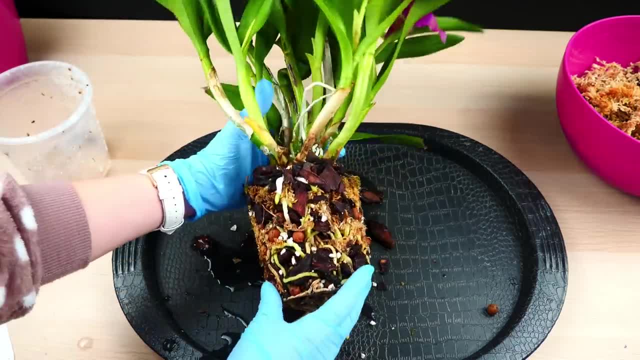 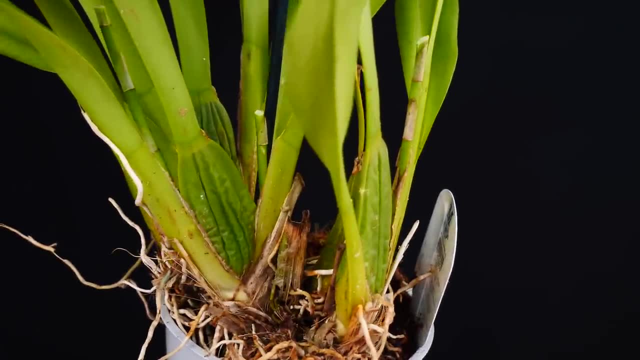 stressing out the plant And in some cases this will lead to transplant shock. Well, imagine if, on top of it all, our orchid is already dehydrated. That amount of stress will make the orchid recover. And if you reduce the dunno power, you greatly diameter the orchid will be less effective any 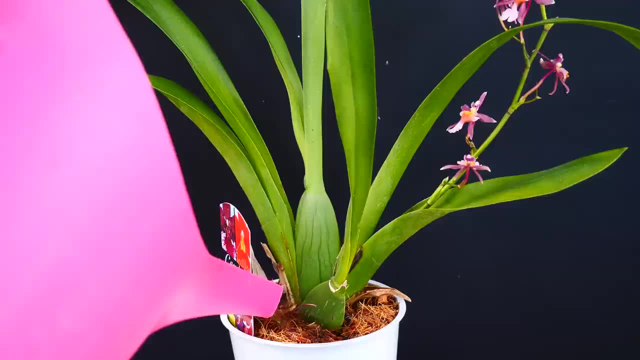 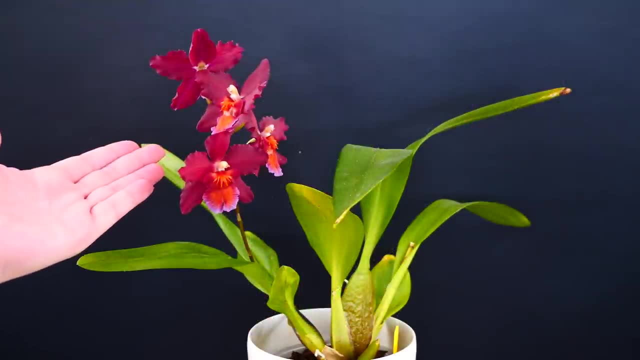 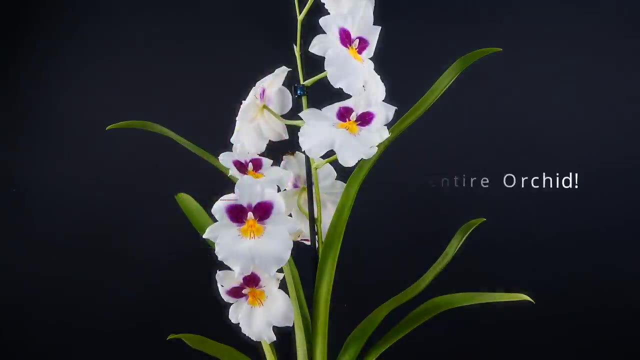 longer. Tip number four: When choosing the pot size, always take into account the entire orchid, not just the root system. Tip on tip number four: Always use a completely hydrated orchid, other than a water-stressed one, when choosing the size of your orchid. This is especially important for watery, super dry ρ orchids. Part Esperma Prospera — for a high- productivity orchid. We're squ GPS seeds for green orchids and nourish orchids and lower risk for flora astrof JAMAаша If you leave your orchid for long periods of time in your garden. 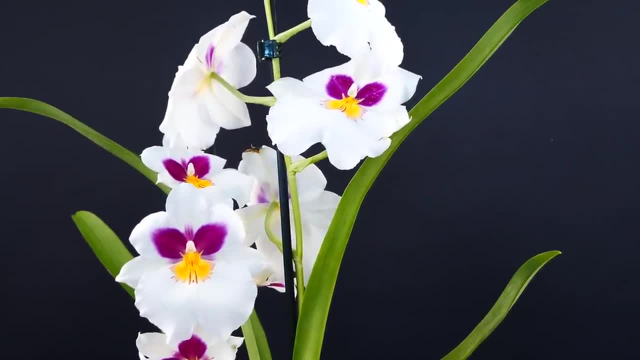 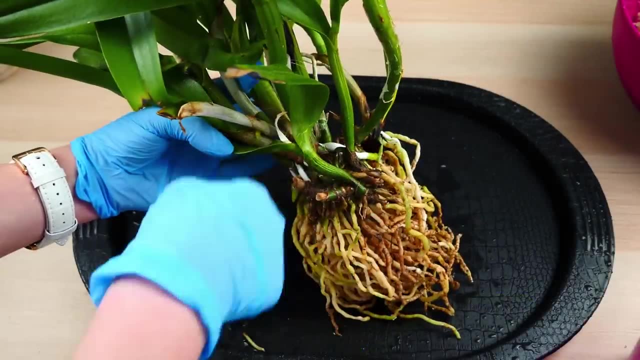 is especially important when dealing with sympodial orchids such as Catleas, Oncidiums and other orchids which produce pseudobulbs or canes. Sometimes you can have an orchid which lost many of its roots, but the orchid herself is pretty big. It's not a good idea to go for a very 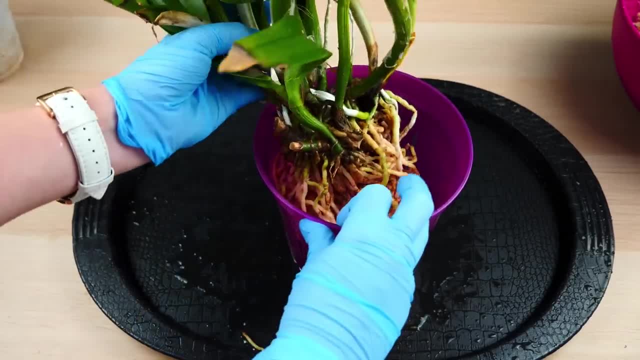 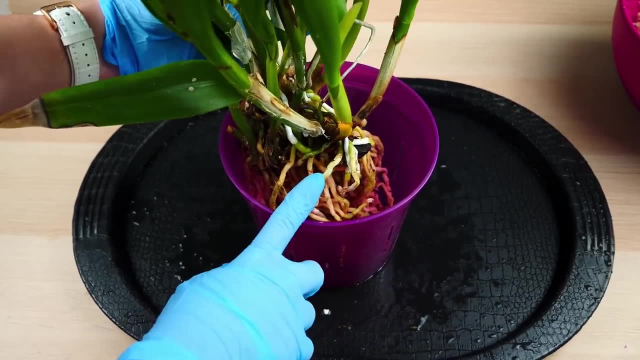 tiny pot which will accommodate the very few roots it has, because in no time the pot will be full of roots and the orchid will have no more room to put out new canes or new pseudobulbs. Find a pot which can accommodate the roots but also leaves a little bit of space for new growth to fit as. 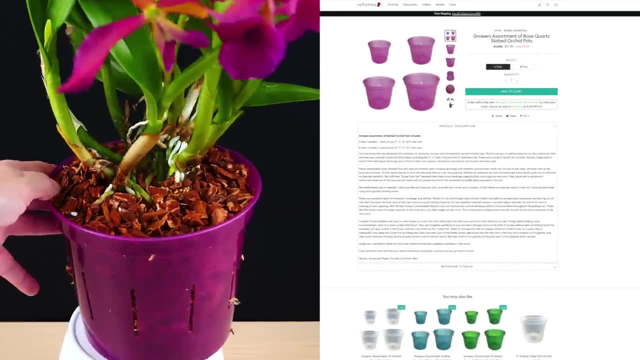 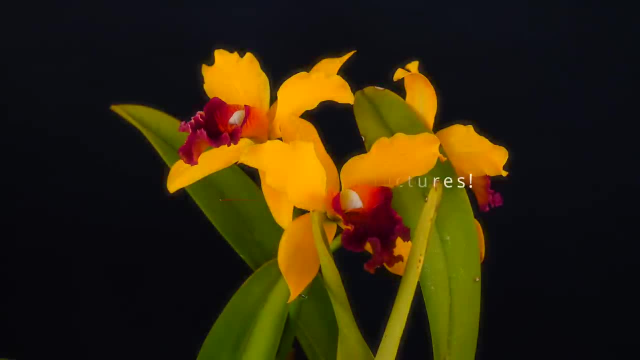 well, So we need a pot which can accommodate the structures. the orchid will grow within two or three years. Tip number five: When repotting older orchids with multiple canes or pseudobulbs, it is absolutely fine to remove the oldest structures. Typically they are the smallest. 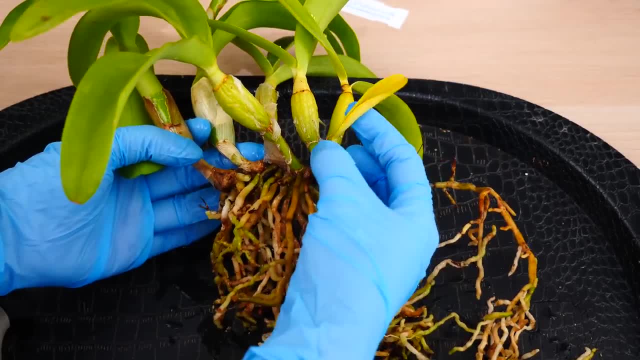 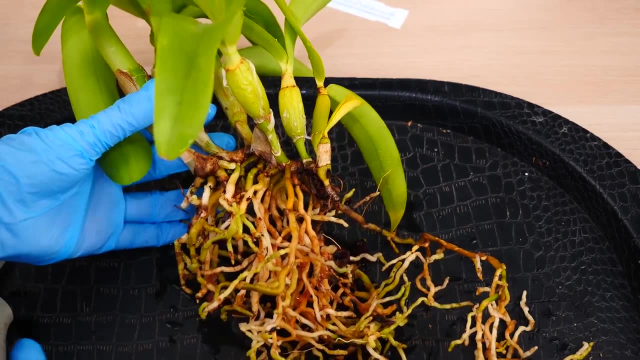 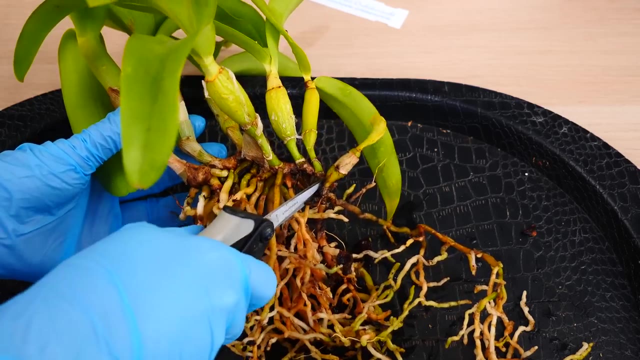 structures on the orchid. In time, these orchids will naturally shed their older structures, Similarly to how Phalaenopsis orchids regularly shed older leaves. very old canes and pseudobulbs will, in time, yellow and dry off. So when repotting such an orchid it is absolutely fine to remove these. 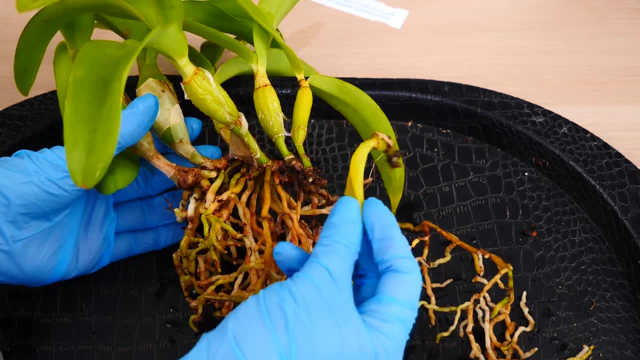 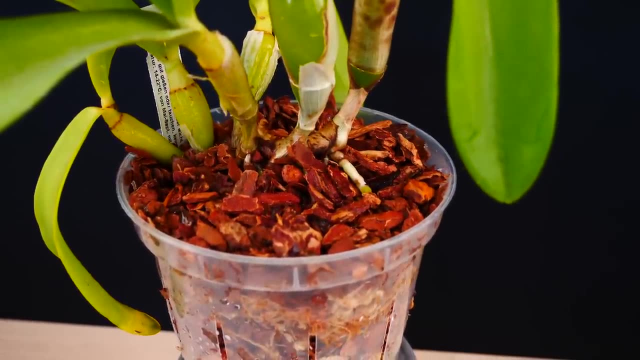 very old structures because they will not last all that much on the plant anyway. The benefit of doing this is that you can actually position the orchid much better in its pot. We can make sure that the newest structures, from which new growth will appear, are positioned as close to the middle. of the pot as possible. So when repotting such an orchid it is absolutely fine to remove these very old structures. Typically they are the oldest structures on the orchid. So when repotting such a new structure, from which new growth will appear, are positioned as close to the middle of the pot as 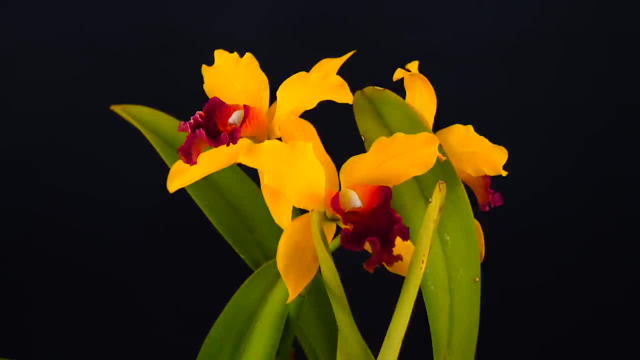 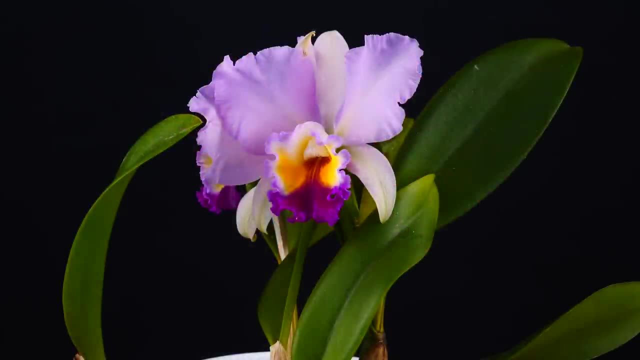 possible. This will extend the life of the orchid in that particular pot and in that medium and limit the number of times we need to disturb the roots. Tip number six: Sometimes you will have to repot orchids with a lot of roots and trying to find all of the dead roots and cut them away. 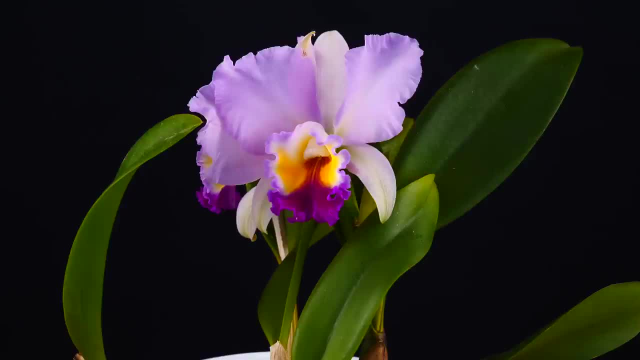 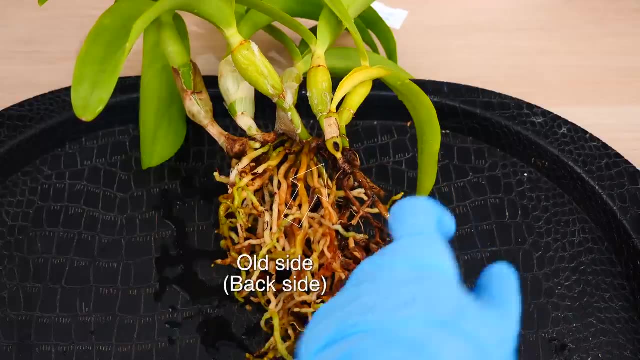 might be a bit of a hassle. Well, you can start by looking at the very oldest part of the orchid. The oldest canes or pseudobulbs will have the oldest roots as well, and the older roots are the more chance you will have of them. So if you have a lot of orchids, you can repot them with a 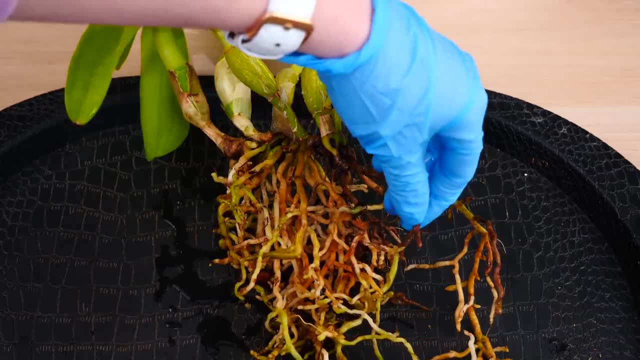 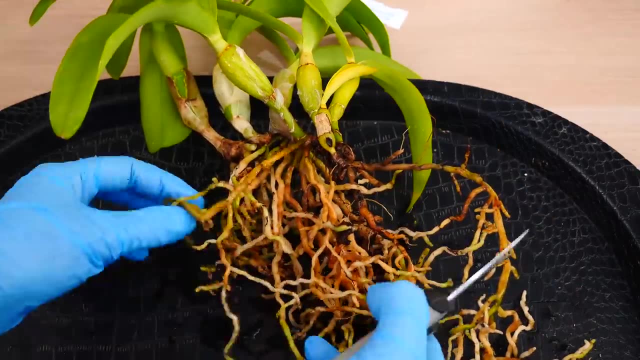 they have to actually not be very healthy or even alive anymore. So start with your search there. Chances are, the vast majority of dead roots are coming from those very old structures. This can actually save you from having to detangle all of that root mess in order to trace back all of the 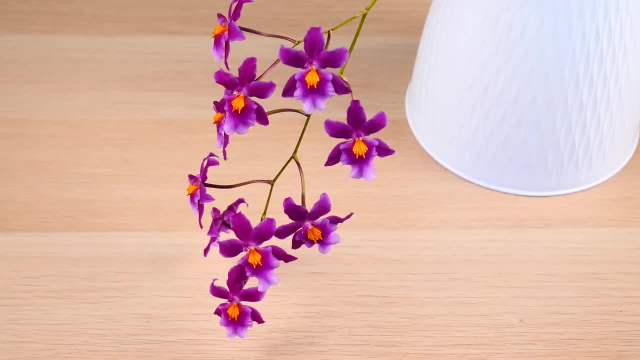 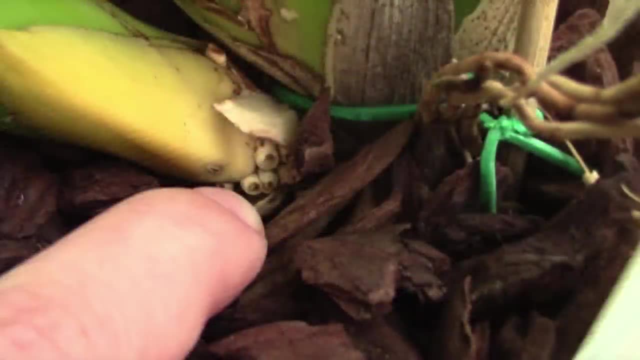 dead roots and cut them away. If you've ever had to deal with those tiny little pesky snails that keep munching on the roots or new growths, well, there is a solution that can be applied during repotting, And this is: Tip number six: If you have a lot of dead roots, you can repot them with a lot of roots. So if you have a lot of dead roots, you can repot them with a lot of roots. So if you have a lot of. 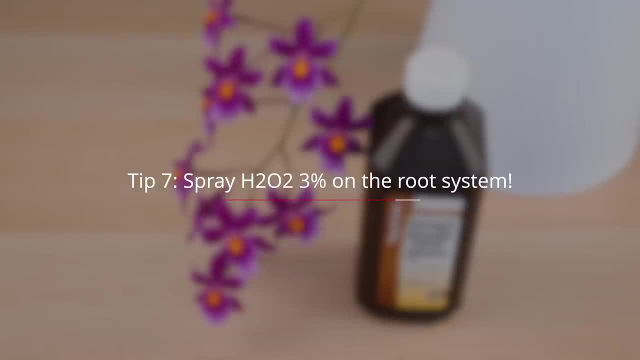 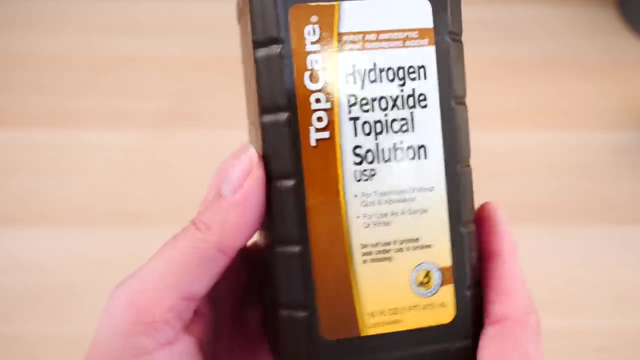 dead roots. you can repot them with a lot of roots. So if you have a lot of dead roots, you can hydrogen peroxide sprays. Hydrogen peroxide can be found at human pharmacies, and the one we use with orchids is the 3% concentration which can be sprayed directly onto the root system. All you 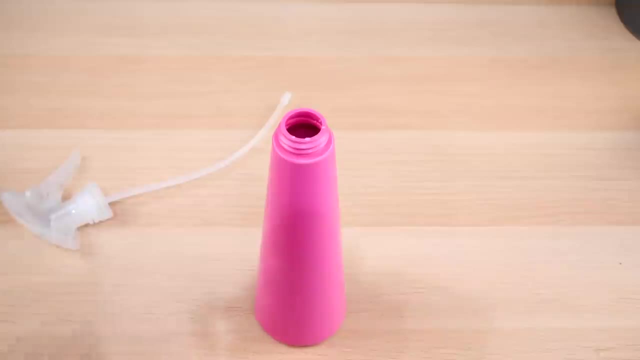 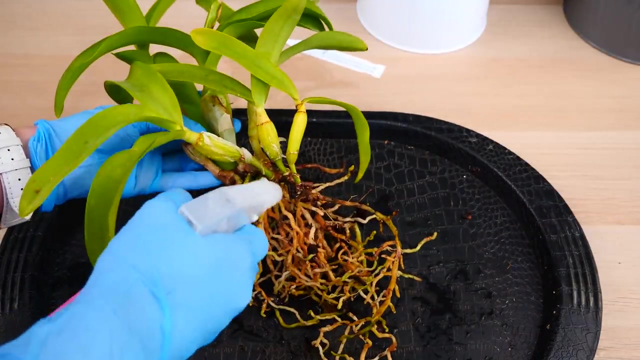 have to do is pour it into a spray bottle and whenever you repot a brand new orchid, after removing the medium and rinsing the root system, you can spray the entirety of the root system with the hydrogen peroxide 3%. This will get you rid of all of the bush snails. 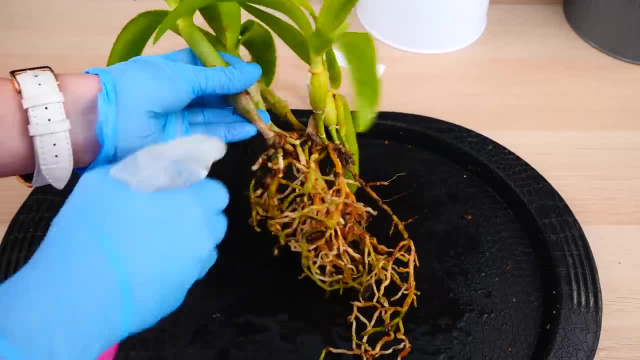 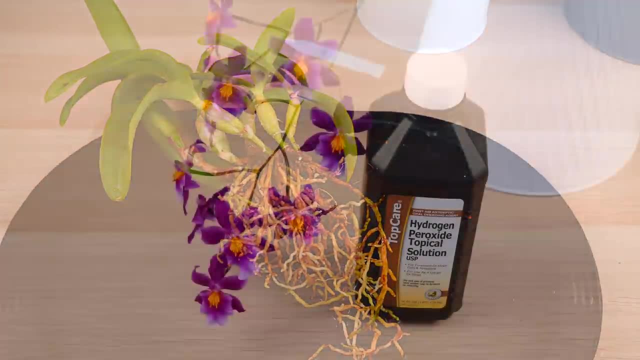 and all of their eggs as well. As a personal note, I had major, major issues with bush snails in the past. I lost many orchids due to them, So whenever I repot a brand new orchid that I don't know, 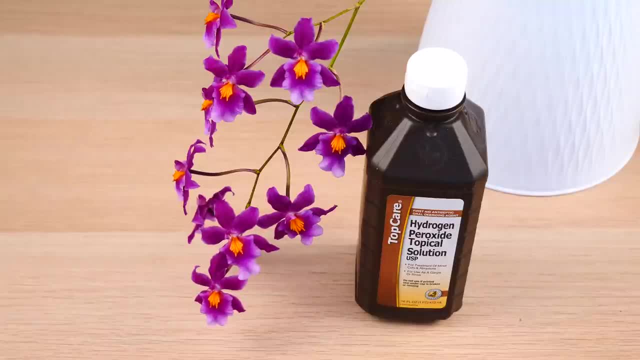 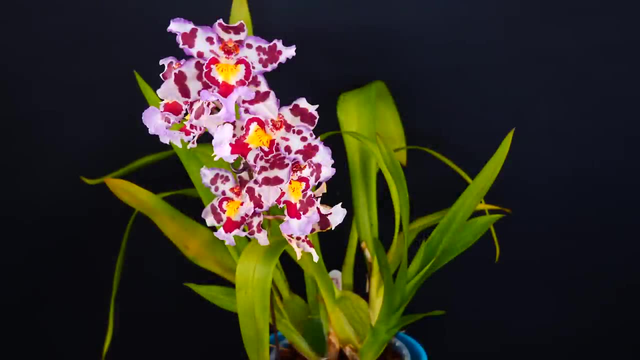 anything about. I always spray the root system And seven years later since I started to use this, I've never had bush snail issues again. After repotting with some orchids, you will discover that they will be rather wobbly and very unstable in their pot. This happens especially. with orchids which last for a long time. So if you have a lot of dead roots, you can repot them with the hydrogen peroxide 3%, Instead of compressing down on the medium and risking damaging any remainder root or removing all of the air pockets. a good tip is to stake your orchid. 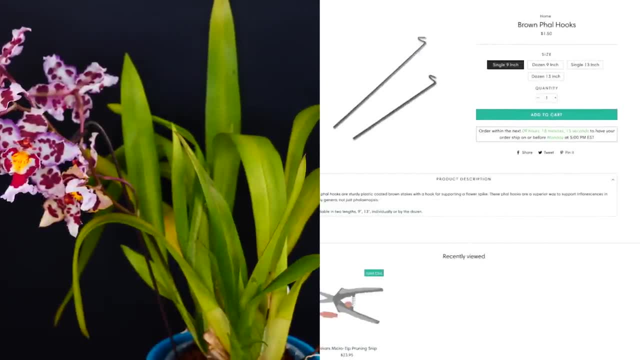 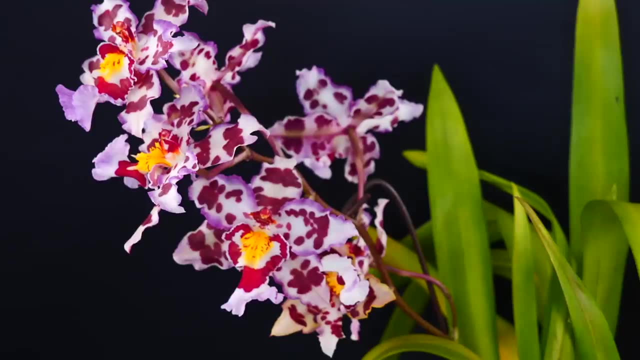 If your orchid happens to have a flower spike, even if it's dry, you can use it in order to stabilize the orchid by staking it, Even if dry and spent flower spikes are still attached very strongly to orchids, so they will keep it in place. 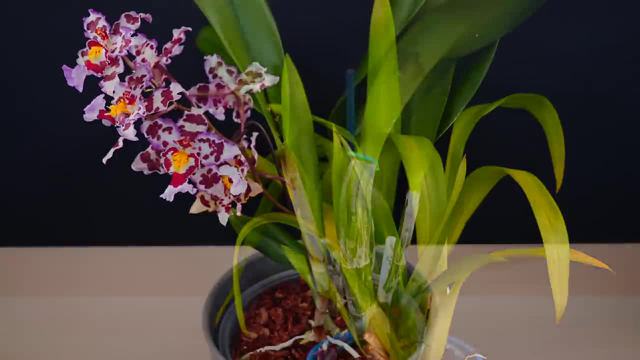 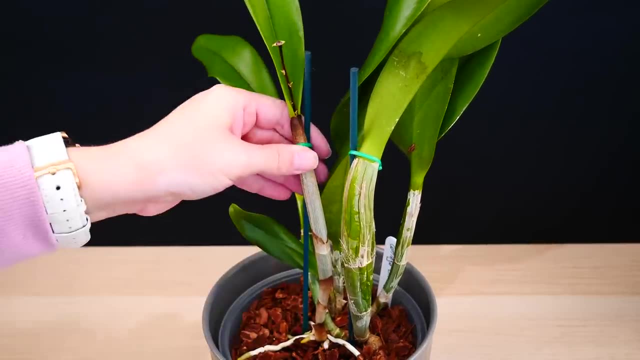 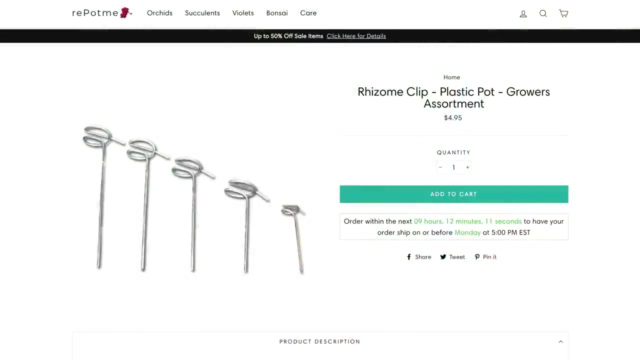 If your orchid doesn't have a flower spike, you can stabilize it by pinning the actual canes or the top of the pseudobulbs to stakes. After the orchid produces roots and stabilizes, you can absolutely remove the stakes. You can also use rhizome clips for orchids which have rhizomes. 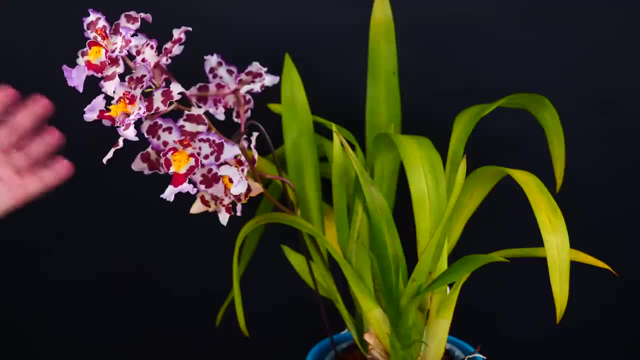 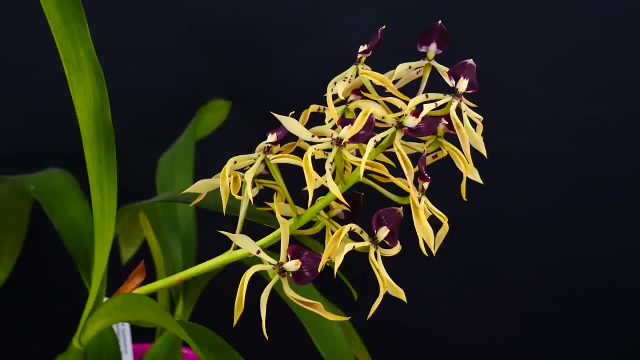 There are many options to consider and in this way you don't have to compromise the airiness of your medium, which is very, very important for any epiphytic orchid. Tip number nine: try to minimize transplant shock. Orchid roots have a tendency to adapt to whatever type of environment. 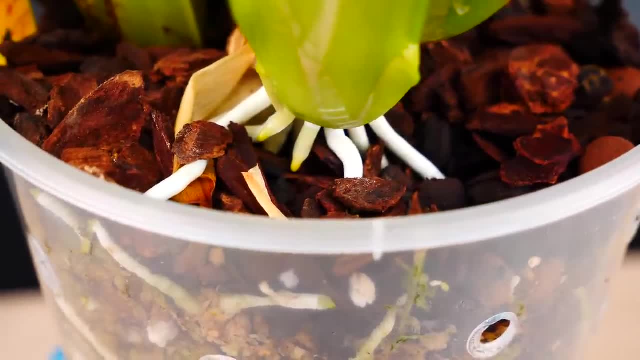 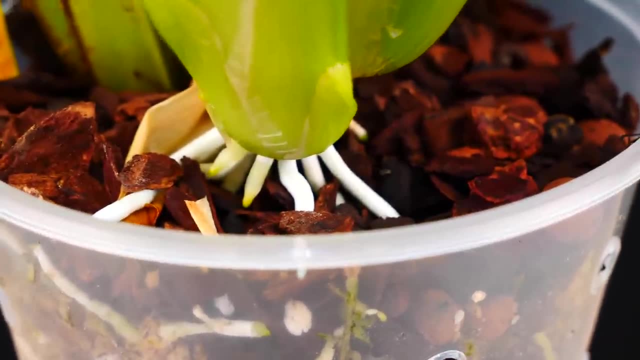 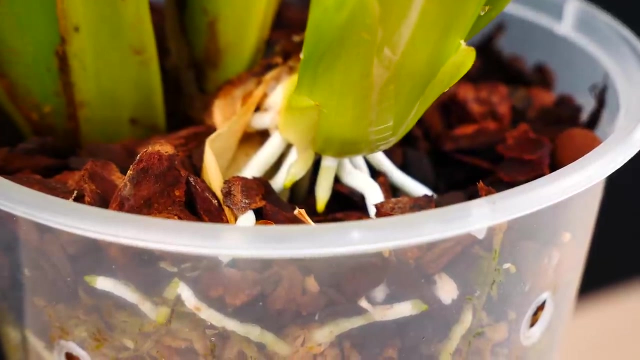 they grow in Meaning. if an orchid has been grown in a very water-retentive medium, the roots are used to high levels of moisture, And vice versa. if an orchid has been grown mounted or in a very, very airy medium, the roots will be adapted to very low humidity conditions and lots of air. 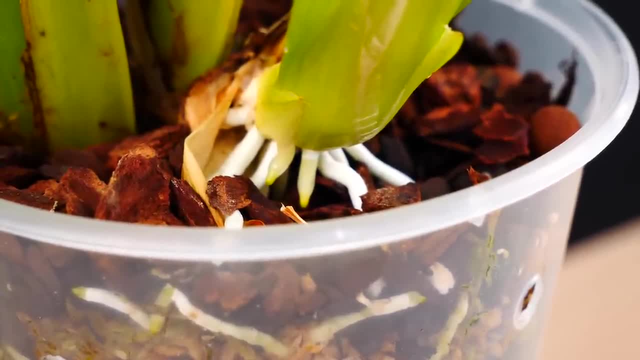 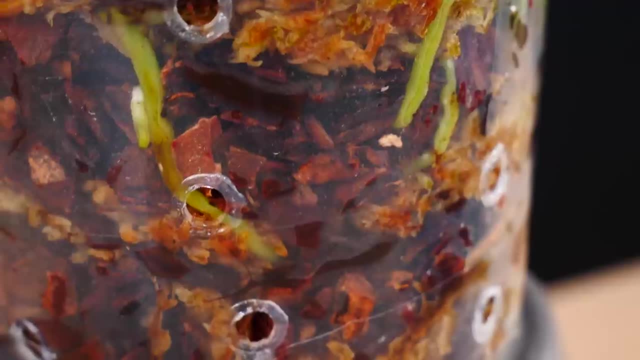 If we try to suddenly change this environment, many of the times the roots will simply die off. For example, if an orchid is potted in pure sphagnum moss and we try to pot it in very airy bark, the roots will not appreciate the fact that they will dry out very fast and most of the times they 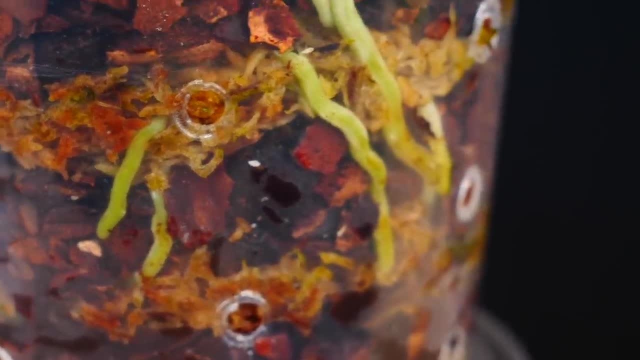 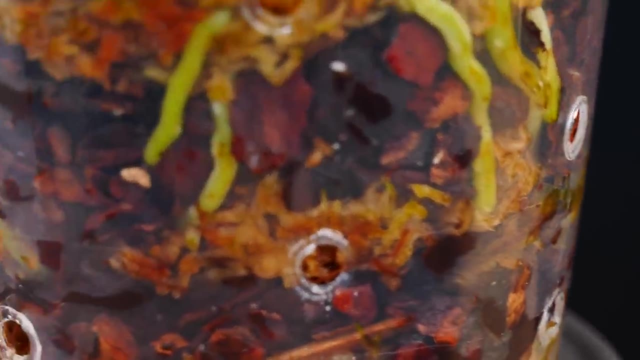 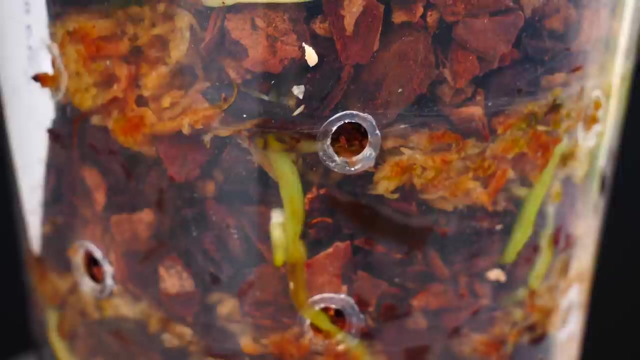 will just wither off. The same can happen for the reverse situation. So the best thing to do when switching from such different media is to try and baby a little bit the existing roots. If you repot your orchid from full sphagnum moss to bark medium, make sure that you do not let those roots 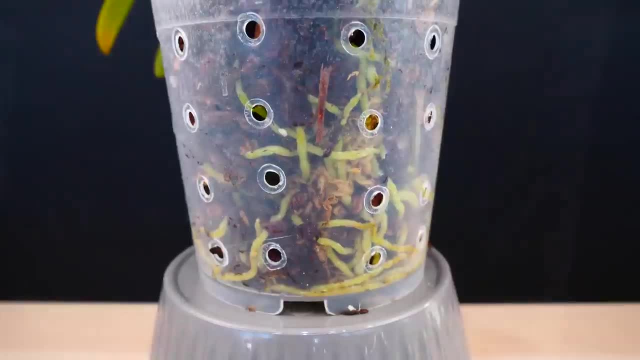 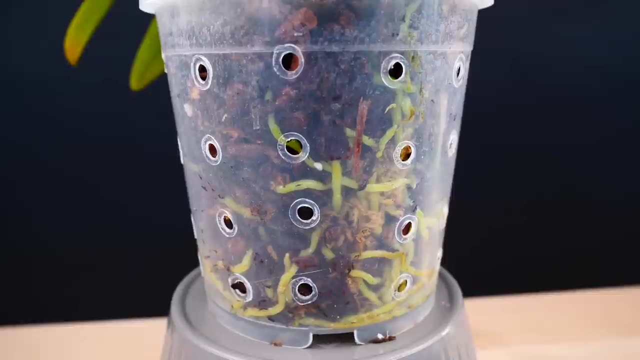 completely dry out, because they won't appreciate it. Try to water your orchid a little bit more frequently just to ease the roots into the new medium. The brand new roots which will grow will adapt to the medium And when they grow big enough you can start watering normally because you will. 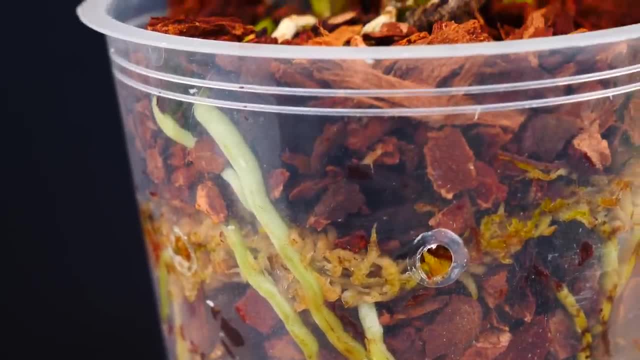 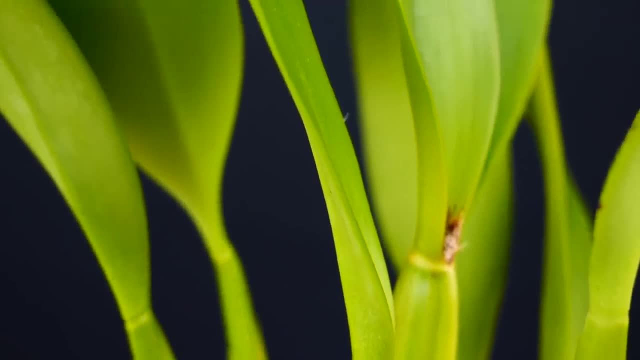 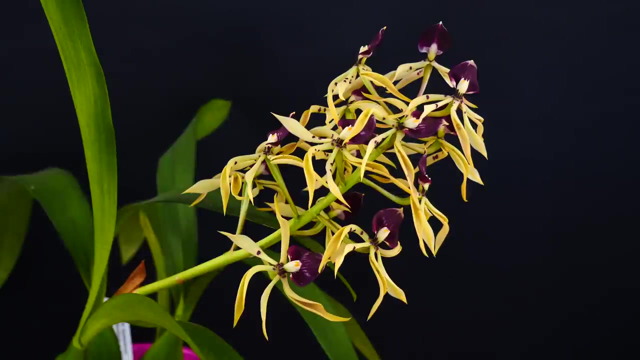 already have roots which are adapted to bark, And the older roots which might end up not adapting will not matter all that much anymore, because we will already have a brand new adapted root system. Until the new root system grows, we can avoid dehydration and stressing our orchid by simply trying to 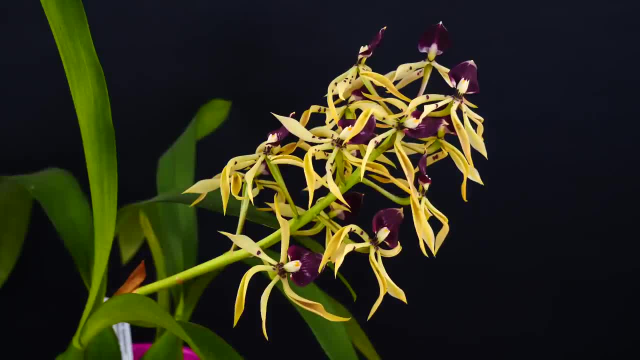 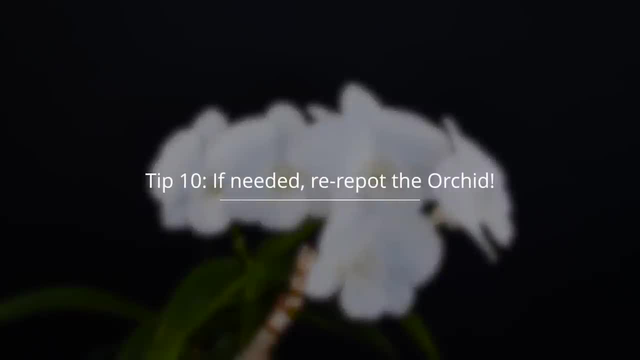 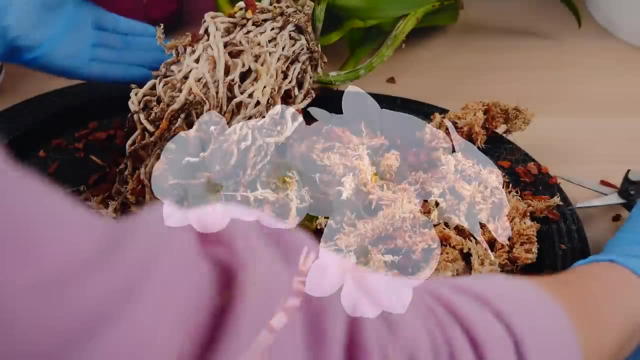 mimic as much as possible. the previous conditions And finally, tip number 10,, which is actually related to the previous tip. In some cases it is actually a good idea to unpot our freshly repotted orchid just to see if we have roots that we need to cut off Now. this tip doesn't. 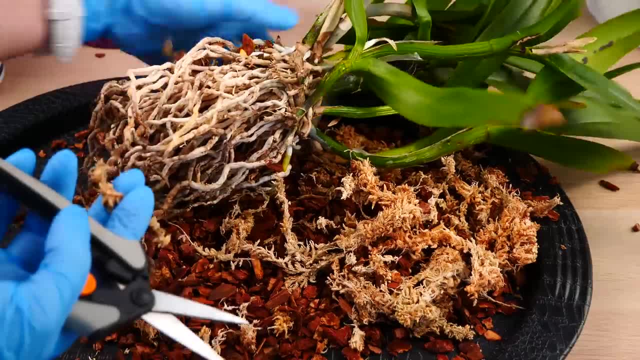 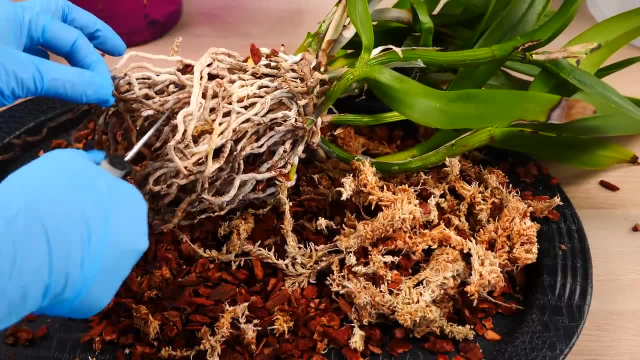 apply to all orchids, but if you know you repotted an orchid with a lot of roots, or an orchid with sensitive roots, such as our cat layout from last month, or you detect a bad smell coming from the fresh new medium, then it's perfectly fine to go back and see if you have any dead roots that you 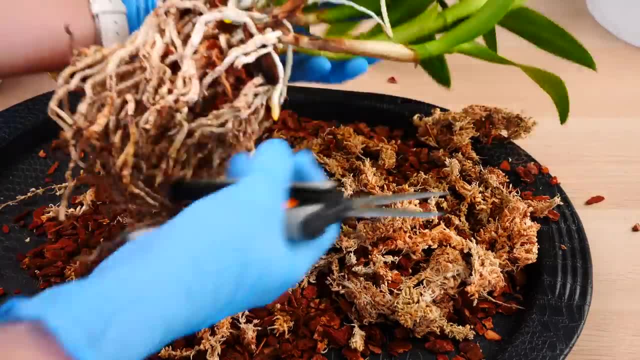 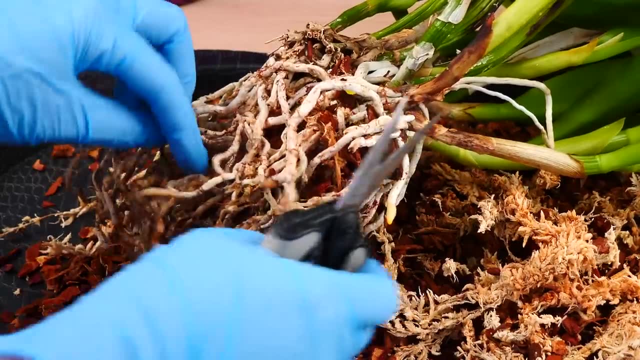 need to cut. Most of the times you will have quite a lot of roots that did not make it. If you repot an orchid with 10 roots and you happen to lose one or two roots, it's not necessary to go back One. 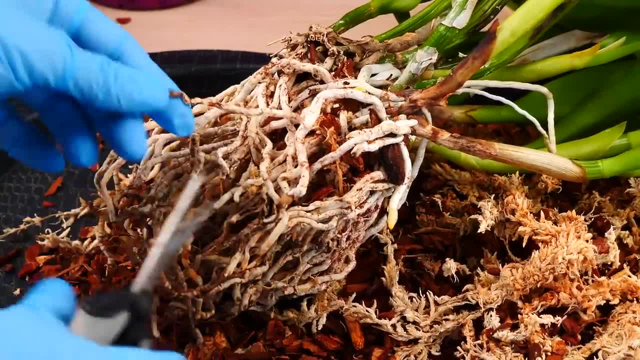 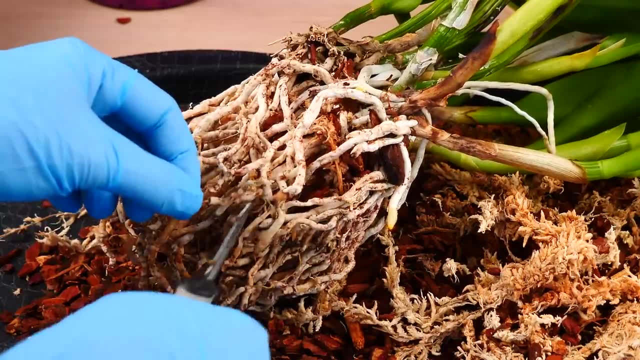 or two roots will not spoil the entire medium, But the more roots your orchid has, the more roots you will have. So in our case, with the cat layout that we repotted last month, we had quite a lot of dead roots to cut away. If I wouldn't have went back and removed those roots in a few months, 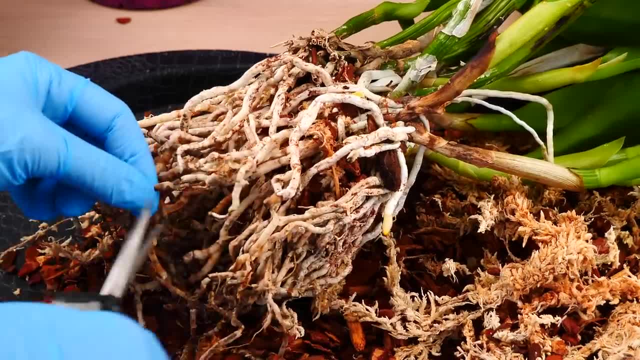 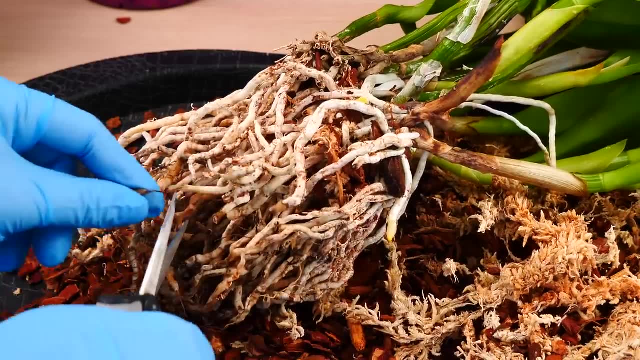 my medium would have already been spoiled and I might have compromised the new roots as well. So be mindful with this tip. Not all orchids will require this. You have to inspect your orchid and try to determine if indeed you need to go back and unpot it In three to four weeks. 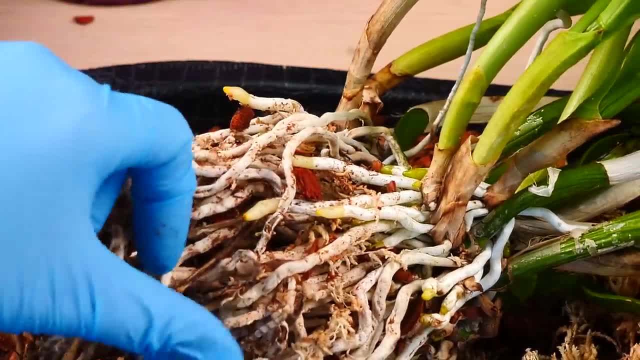 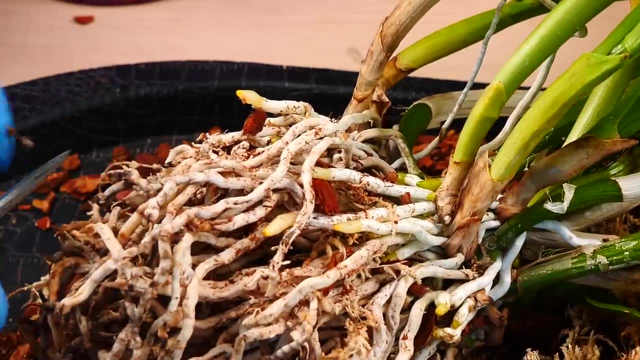 new roots didn't really have time to attach to the sides of the pot, so you will not damage them And also you can definitely reuse the same medium if you make sure to remove all of the debris that the roots left behind. So these have been the 10 orchid repotting. 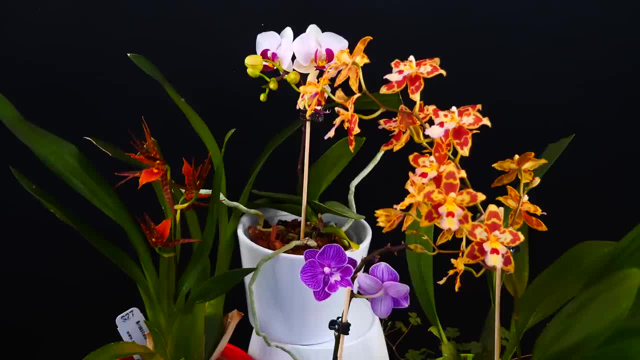 tips that I really hope will make repotting much more successful for you. If you're interested more on how to actually repot orchids, I will link you down below to my extensive guide on repotting Phalaenopsis orchids and also the cat layout orchids care tutorial that we did last month. 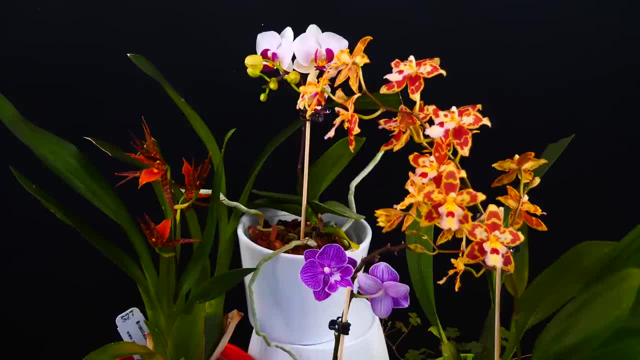 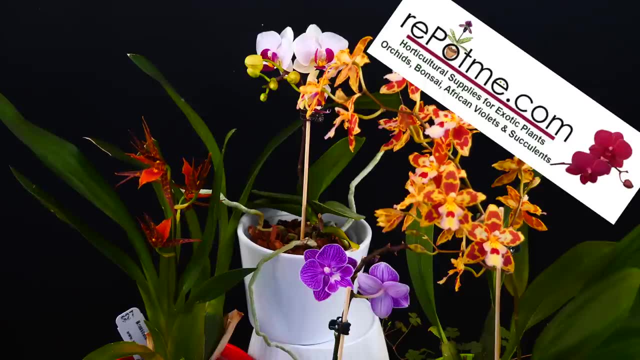 because I repotted cat layout in that video. So if you have any questions, feel free to contact me. And other information that I find useful You'll find it all down in the description. Thank you again, RepotMe, for making this series possible as well.